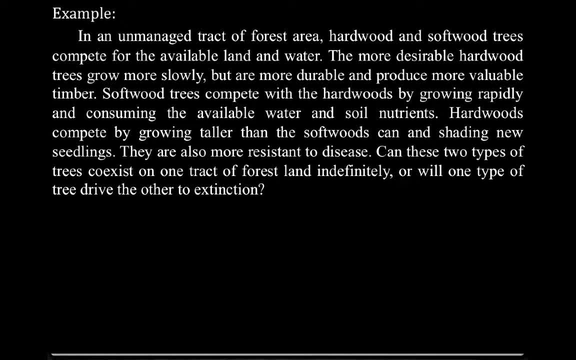 Hardwoods compete by growing taller than the softwoods can and shedding new seedlings. They are also more resistant to disease. Can these two types of trees coexist on one tract of forest land indefinitely, or will one type of tree drive the other to extinction? 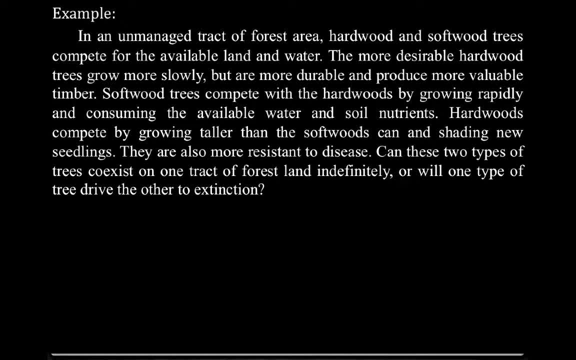 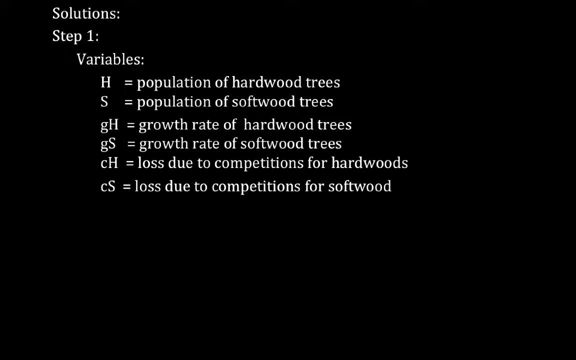 Okay, we will use the five-step method for this problem. Step one is to define variables, assumptions, then decide the objective. Let me go to step one and define variable. We have two populations: Population of hardwood trees and population of softwood trees. So 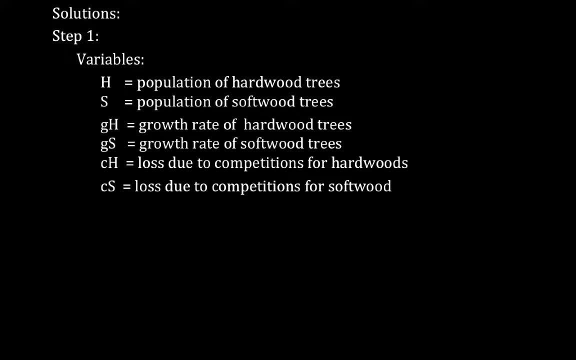 I will take H and S respectively. for those, Then, growth rate of hardwood trees. GH and GS is the growth rate of softwood trees. Finally, we will take CH and CS: loss due to competitions for hardwood and loss due to competition for softwood respectively. 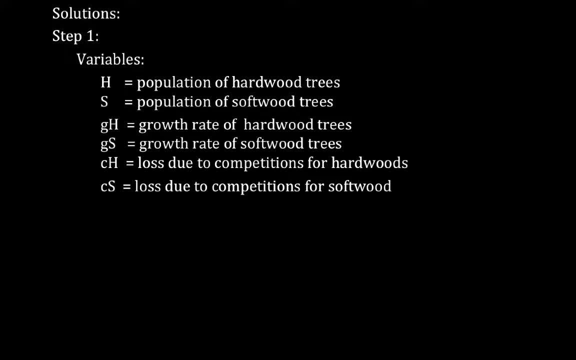 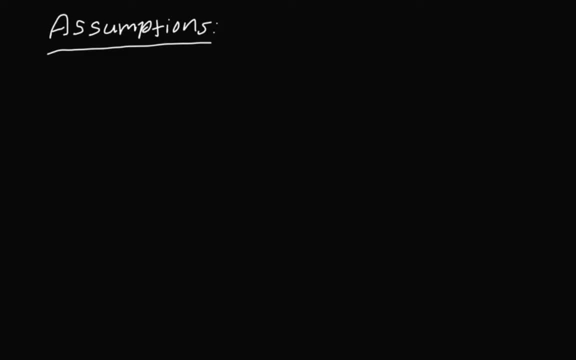 Okay, next, Then we will take CH. What you must know, What you must know, is: what are the things we need to look at to define the byproduct? So one of the things we want to look at is: what is this byproduct? 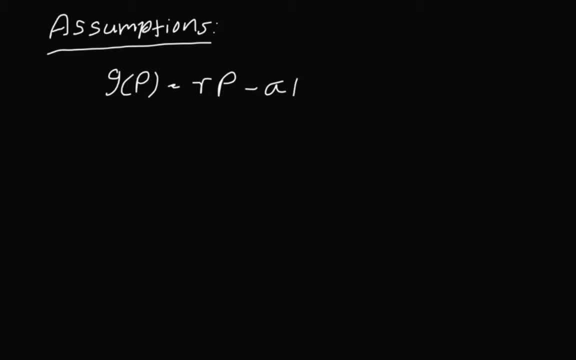 Why this guy? Why this? this guy is like the guy who is helping us find the byproduct of a stream. Question is: why? Okay, let us see. So here we know: R is the intrinsic growth rate and A is a measure of the strength of. 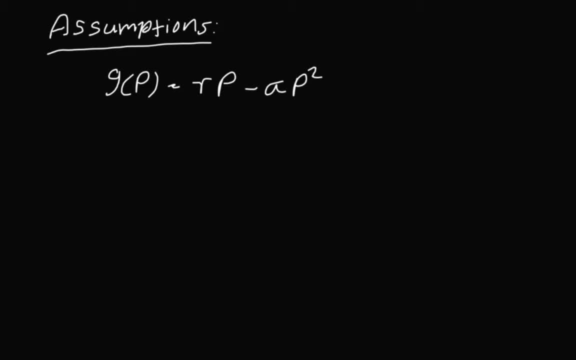 resource limitations, We should use this equation: Gs is the growth rate for hardwoods. so according to this equation, we can write down Gs: R1. population H minus A1 H square H is the population of hardwood. Similarly, we can write down Gs, which is growth rate for softwoods equal R2s minus. 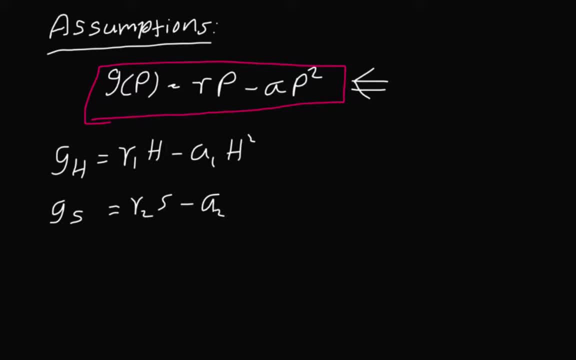 A2, H2, power 2.. According to above equation, so R1, R2, A1, A2 are positive reals. So then we know Ch, which is loss due to competition for hardwoods. So we can write down this: B1, which is a positive real, equal Ch, equal B1 times Sh. 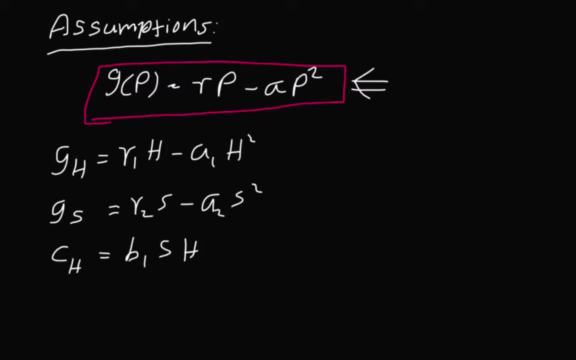 Similarly, Cs can be written b2sh, so b1, b2 are also possible reals. But we know it is very clear: h greater than or equal to 0 and s greater than or equal to 0, for our assumptions. 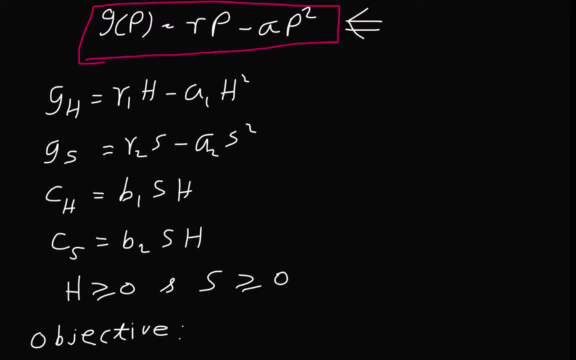 Then we need objectives. objective according to the example. we need to check whether h goes to 0 or s goes to 0. Next, step 2, step 2 is to select the modelling approach. As I mentioned before, we will model this problem. 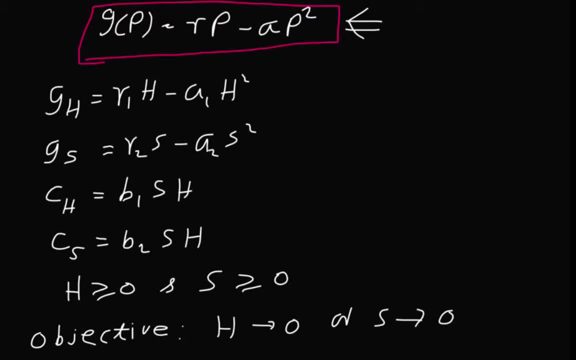 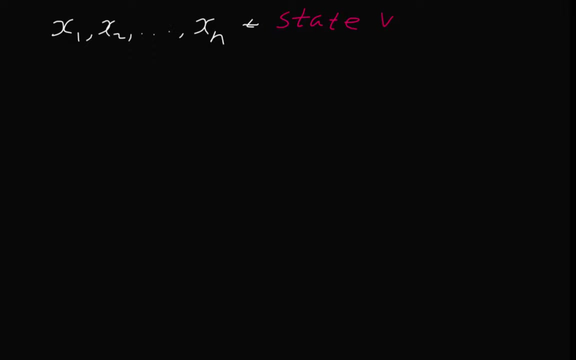 As a dynamic model in steady state. Suppose, we have n variables, x1, x2, xn, So these variables are called state variables. State variables- State variables. We are given functions n functions f1, x1, xn, f2, x1, 2xn. 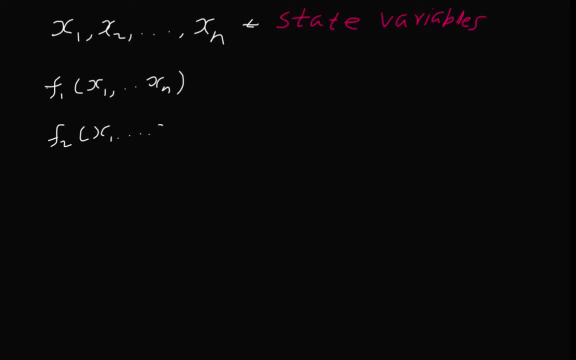 Then fn. x1, xn. 2xn. Then fn. x1, xn. Then fn. x2, xn, x1, xn. These functions represent the rate of change of each variable: x1 to xn, respectively. x1 to xn. it means this is the rate of change of x1,. this is the rate of change of x2,. 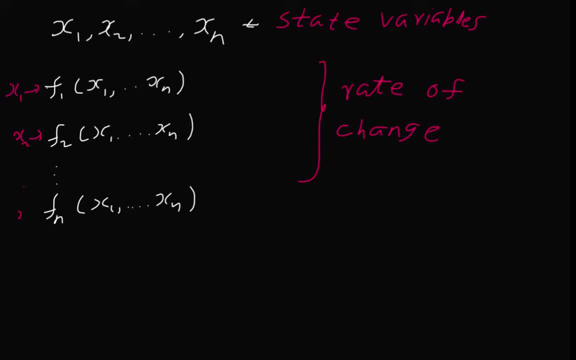 similarly this is for xn. So we can write down a point: x1,, x2,, xn. This is a point in the set S which is called state space. So again, understand, we do have n variables, which is called state variables. Then we have functions. 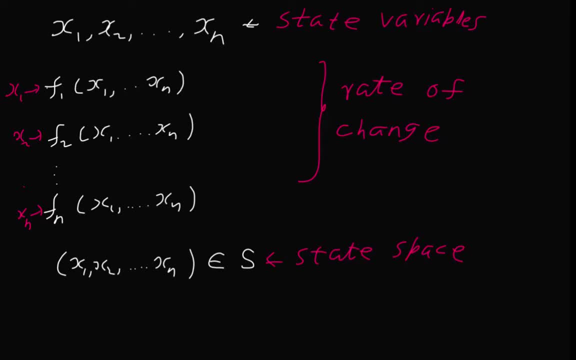 f1 to fn represent the rate of change of each variable, x1 to xn respectively. Then we can find, we can write a point x1, x2, xn which is in the set S which is called state space. Then point x1, x2, xn is called an. 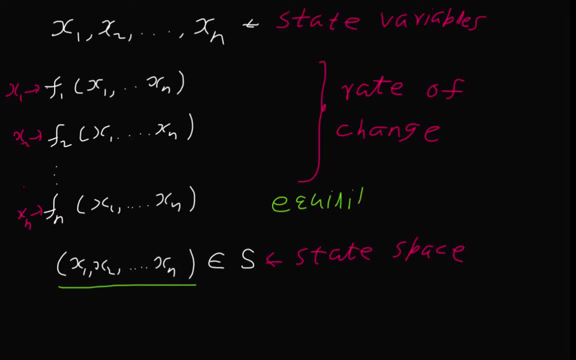 equilibrium point. Equilibrium point: It's a point provided that f1 equal to 0, f2 equal to 0, fn equal to 0. When we are at an equilibrium point, we say that the system is in steady state. At this point, all of the rates of change are equal to zero. For this reason, these equations are sometimes referred to as the balance equations. 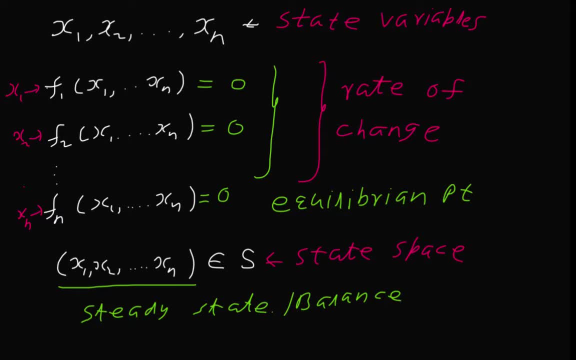 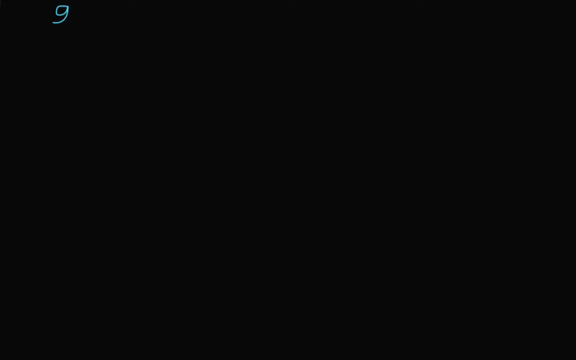 Balance equations. This is the step 2.. Now step 3.. Step 3 is to formulate the model. Now go back to the assumptions in step 1.. So we write some equations: GH is growth rate for hardwood And GS is the growth rate for softwood. And CH CS? 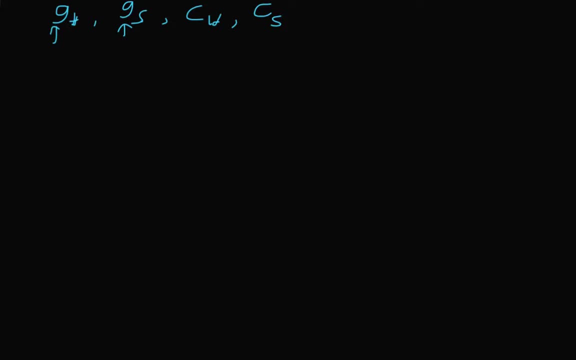 CH lost due to competition for hardwood And CS lost due to competition for softwood. Let's calculate X1 equal H and X2 equal S. Then we can write down GH using X1 and X2 are 1, X1 minus A1, X1 to power 2.. 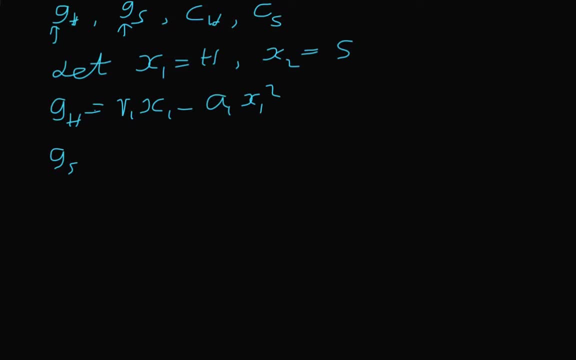 So GH R2, X2 minus A2, X2 to power 2. CH B1, X1, X2 and CS B2, X1, X2.. Here we do have two variables Instead of any variables in a step 2. 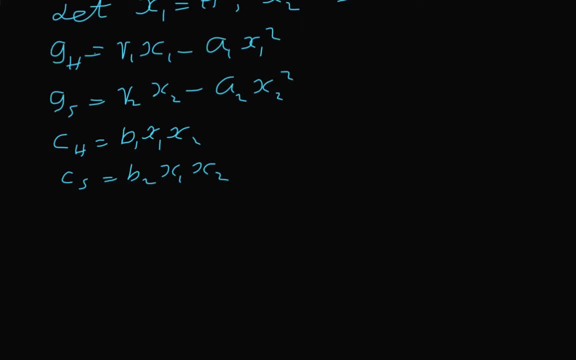 X1 and X2 are the two variables. Therefore, I can define a point: X1 comma X2, there's a point, And So let me, So let me define a set, then: x1 greater than equal 0, x2 greater than equal 0. so this is the s we can. 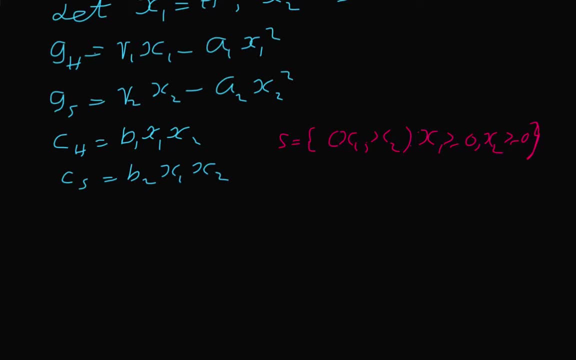 write two functions because we do have two variables. therefore we must have two function: f1, x1, x2. this can be written. what is f1 first? f1 represent the rate of change of variable x1. so how do we write down this? gh, which is growth rate for hardwood minus. 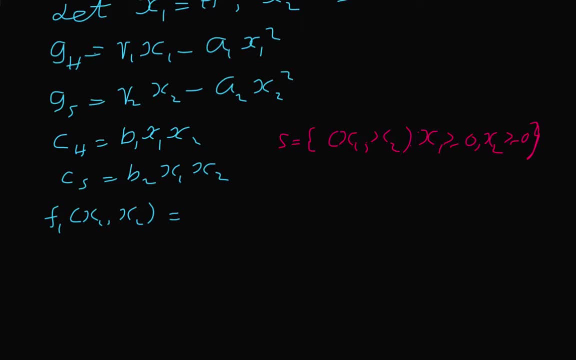 loss due to completion for hardwood, which is ch. i mean if i write down in notation: gh minus c, m star: 1 x1 minus a1, x1, square minus grwell, b1 x1, x2.. Similarly you can write down for the f2: x2.. Now we do have two equations. Next set these: 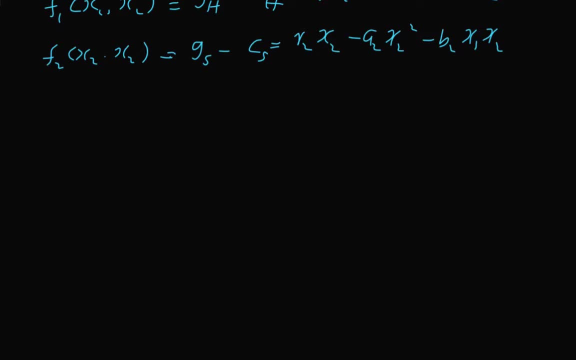 two equal to zero, which is r1- x1 minus a1, x1 minus b1, x1- x2 equals zero. This is the one we discuss under step two: f1- x1- x2 equals zero And similarly, f1- x1- x2 equals zero. 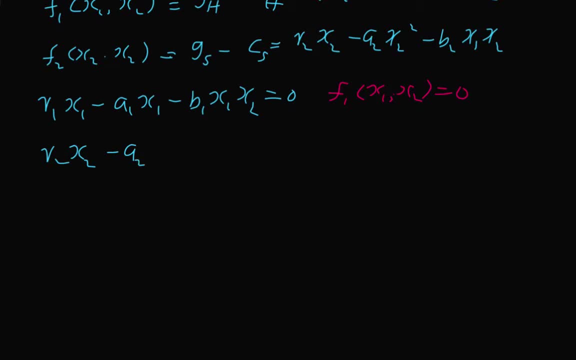 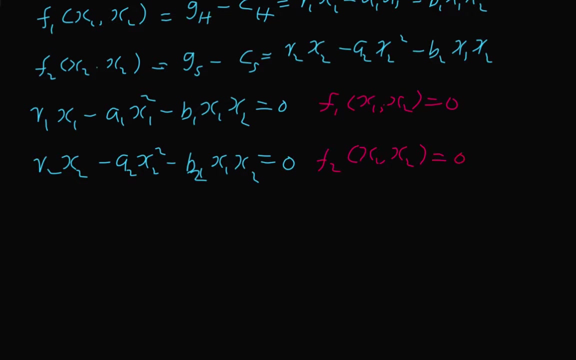 r2- x2 minus a2- x2 squared. Actually, this should be squared Minus b1- x1- x2.. I'm sorry, this should be. b2 equals zero. This is the one. f2 x1- x2 equals zero. Now solve for x1 and x2.. 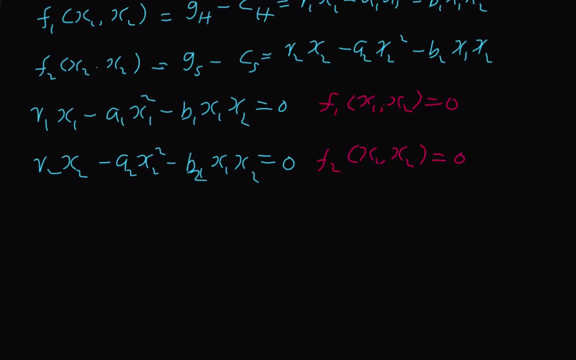 Let me name these two equations Call: this is first one and this is second one. So first one. you see, x1 is the common. The factors are r1 minus a1, x1 minus b1, x2 equals zero, And second one, X2 can be taken out. then R2 minus A2, X2 minus B2, X1 equals 0. 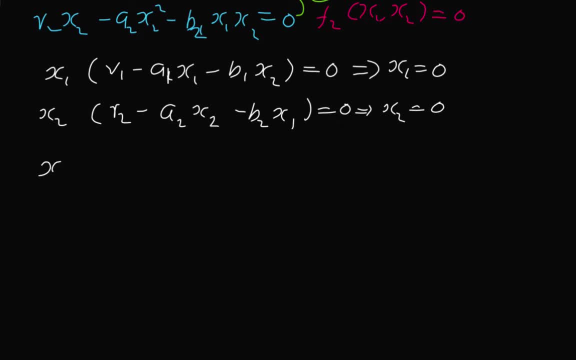 For the first equation you get: X1 equals 0, R1 minus A1, X1 minus B1, X2 equals 0.. So second one: X2 equals 0, so R2 minus A2, X2 minus B2, X1 equals 0. 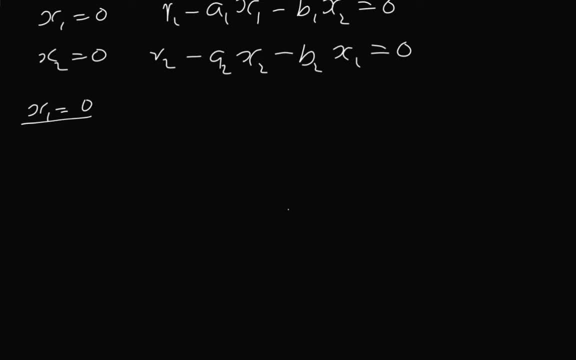 When X1 equals 0, we can plug the X1 value to 0. So this equation: so then you will get X2 equals R2 divided by A2.. Therefore we have a point 0, R2 divided by A2, then X2 equals 0. 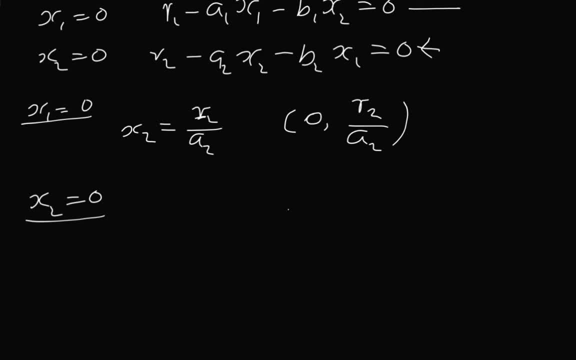 So you can plug the X1 value to 0.. So then you will get X2 equals 0, R2 divided by A2, then X2 equals 0. So you can use this equation: then R1 minus A1, X1 equals 0. 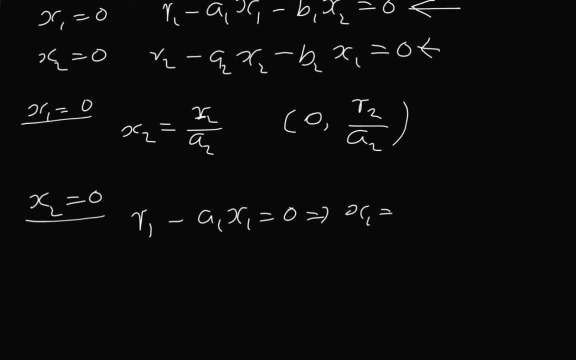 From here you can say: X1 equals R1 divided by A1. So the point is 0,, I'm sorry, not 0. So point is R1.. So now we do have two points, the first one and the second one. 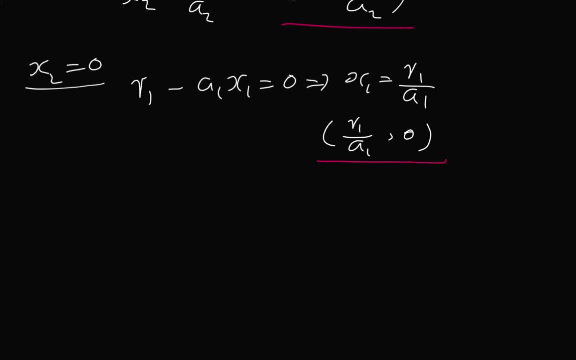 Not only these two points. and you see, we do have 0, 0, so we should consider 0, 0 also. There's a next point, third point: Not only the three points, we have one more. How do we find it? 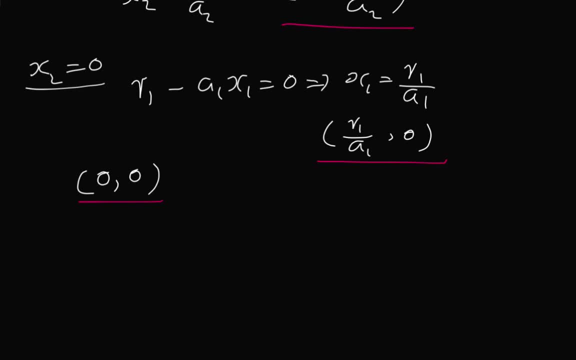 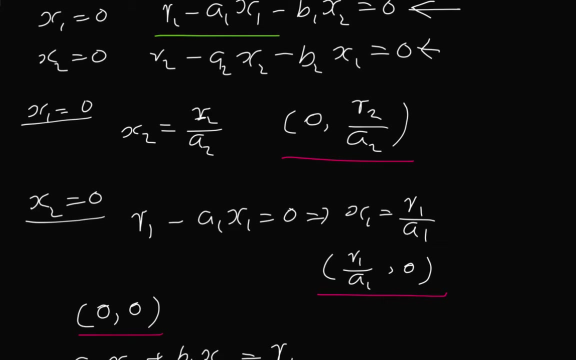 Okay, you see We have two equations. It means A1, X1 plus B1, X2 equal R1.. If you see this one, let me show you this equation. I can get the equation I just wrote. Similarly, consider this equation. 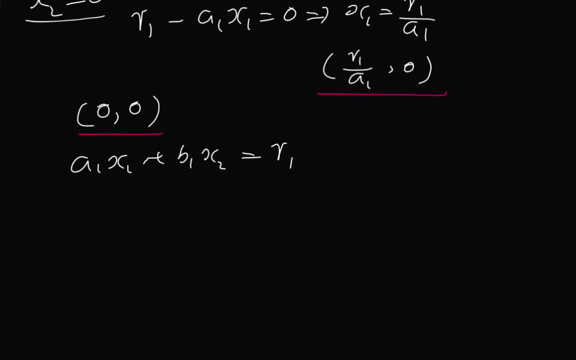 So let me write down the equation for that. So B2, X1 plus A2, X2 equal R2.. Now solve these two equations for X1 and X2.. You know how to solve it, So you can get it. 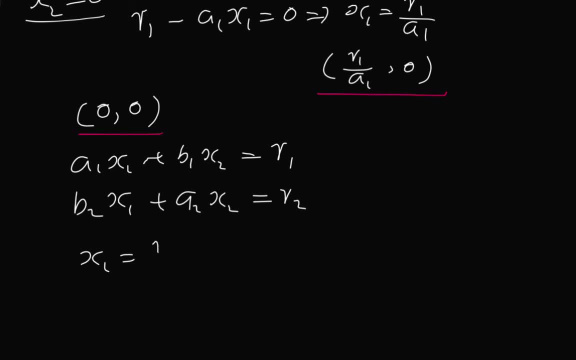 X1 equal R1, A2 minus R2.. B1. B2 equal R1 divided by A1, A2 minus B1, B2.. And X2 can be written: A1, R2 minus B2, R1 divided by A1, A2 minus B1, B2.. 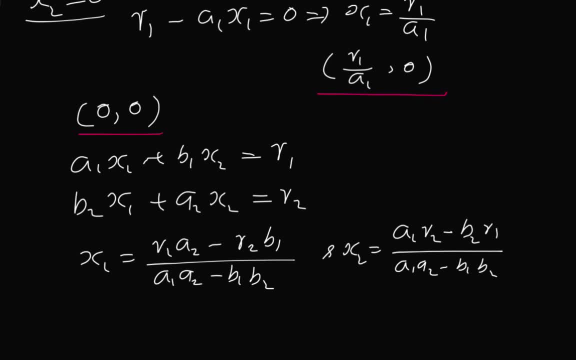 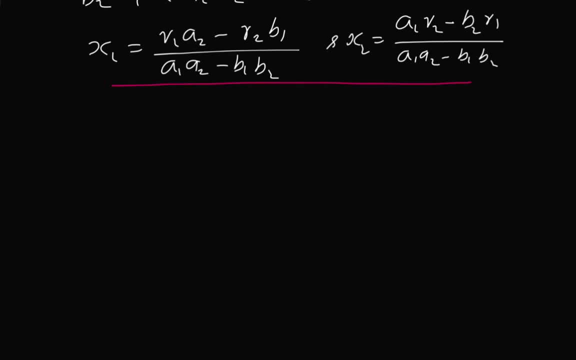 So that is the X1.. And X2 for the last point. So we do have actually four points. Now, if we draw a graph, you will see. this is X axis, This is Y axis. We have two linear equations. 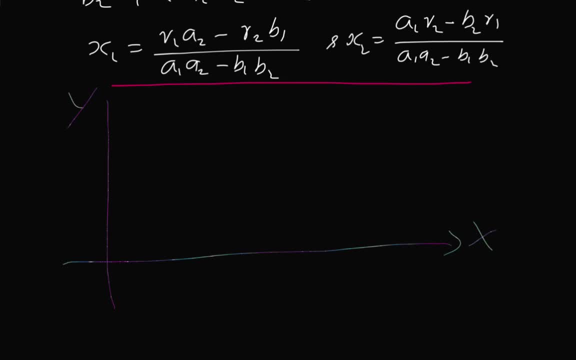 A1, X1 plus B1, X2, equal R1.. And B2, X1. Plus A2, X2, equal R2.. So if we draw these two equations, you will get this one. These are the four points we already have.